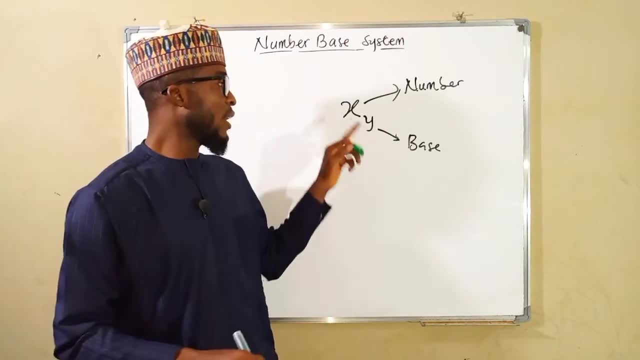 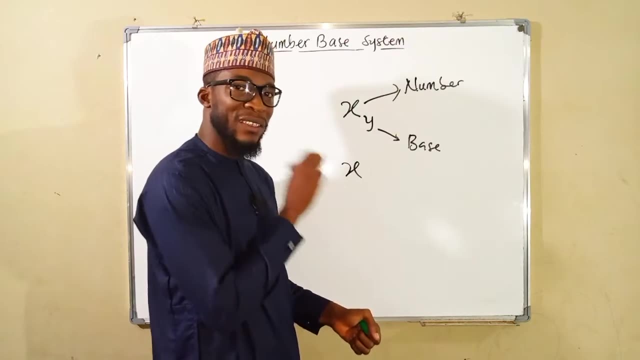 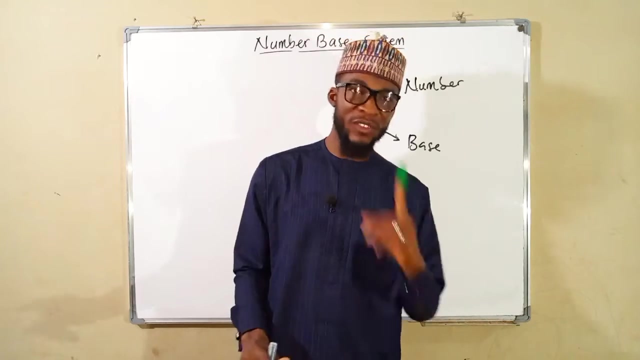 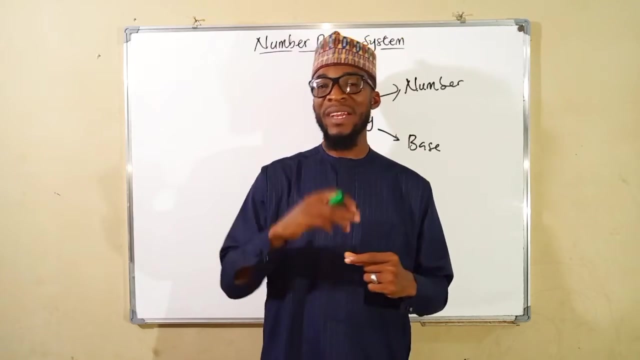 there are two important things you need to know. Any number without an assigned base- suppose we have just x as a number- That number is in base 10, naturally, if it does not contain any assigned base. That's number one. Number two: you need to know that the highest digit in any number base is one. 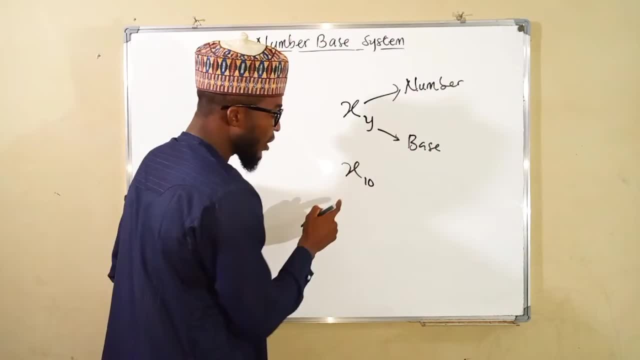 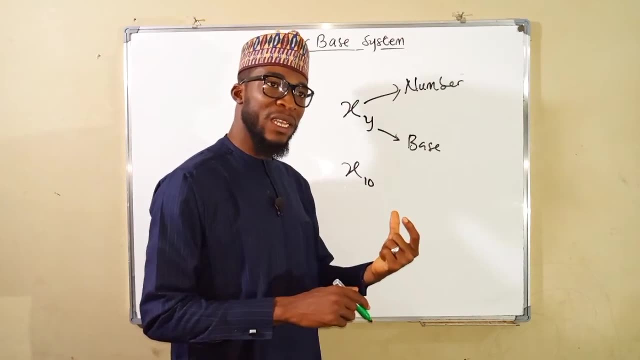 less than the base itself. So if you are talking about numbers in base 10, you will never see 10 within the range. If you're talking about numbers in base nine, you can only see numbers from zero to eight. If you're talking about 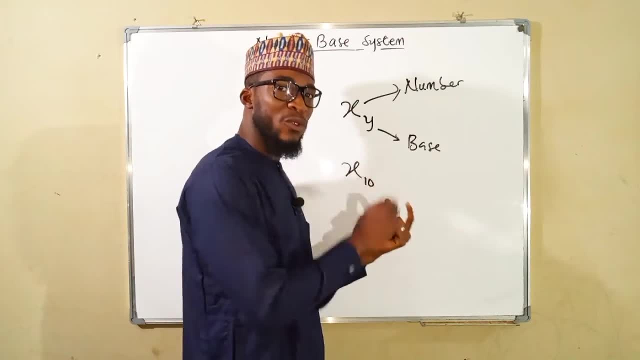 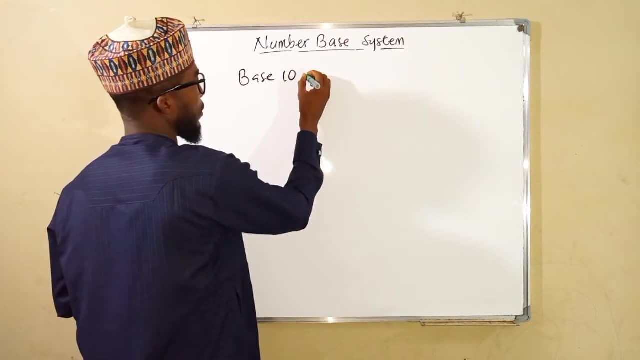 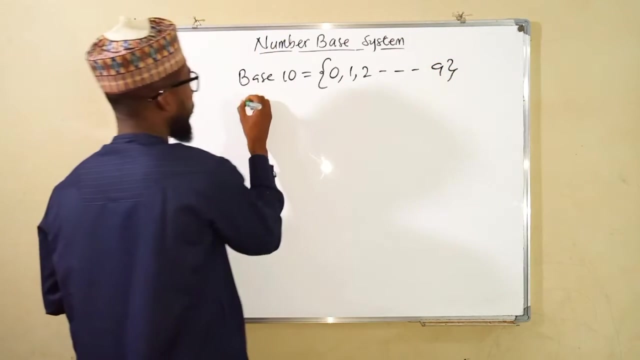 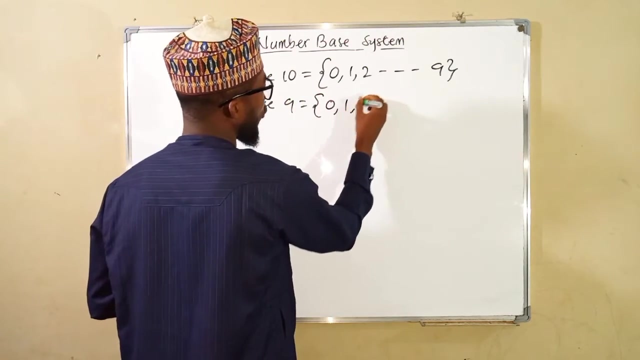 base 7, you can only see numbers from 0 to 6 in that order. So for base 10, the only available numbers there are 0,, 1,, 2,, up to 9.. For base 9, you can see numbers from 0. 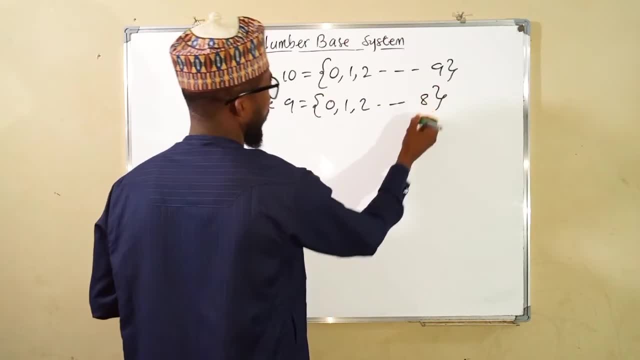 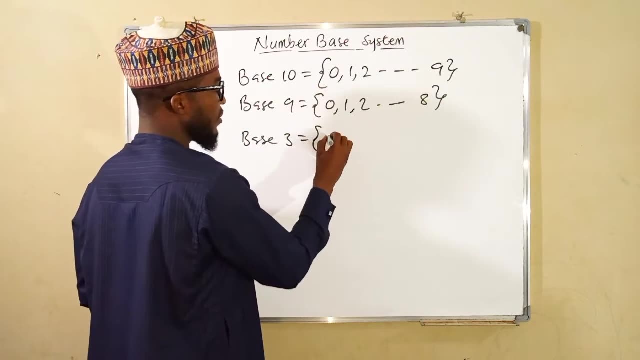 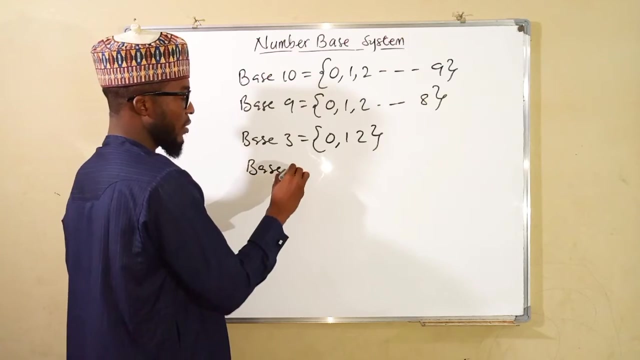 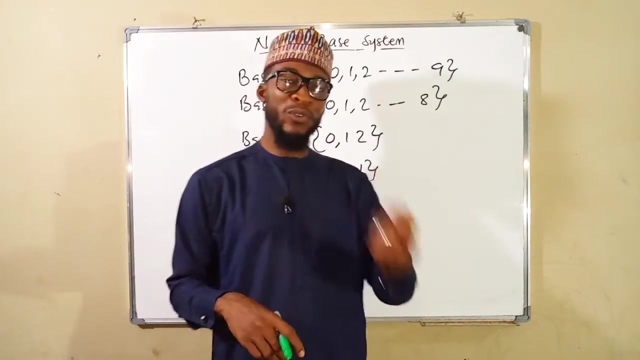 to 8.. If you're talking about base 3, you can only see numbers like 0,, 1 and 2.. If you're talking about base 2, you can only see 0 and 1.. So now let me explain that bundle. Suppose. 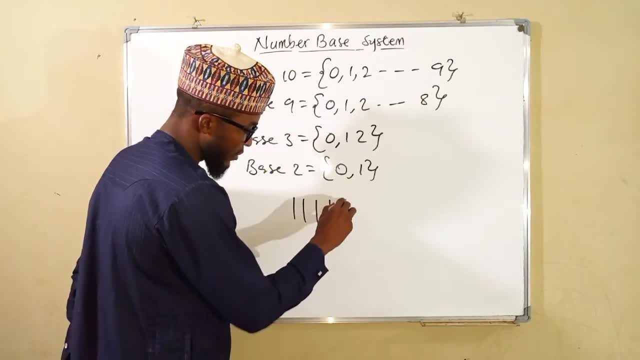 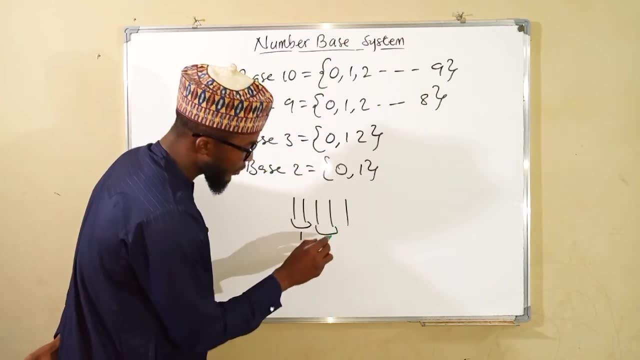 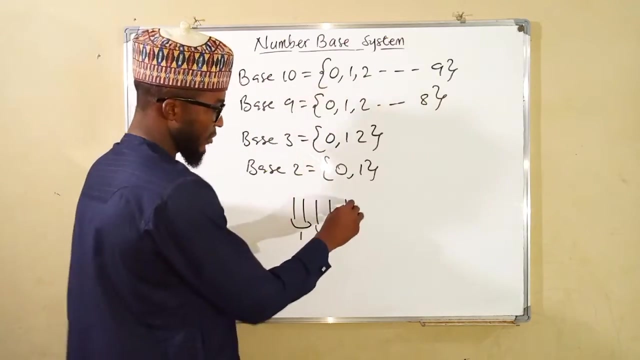 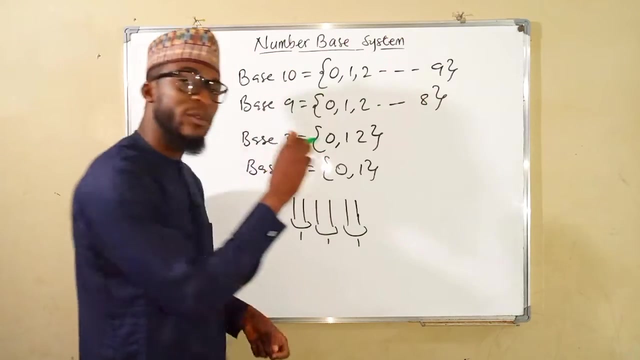 we have five items And we want to group them in two. So every two form a bundle And we have an extra which we call a unit, And if you were to add an extra item, just a single item, that single item is going to be linked off with the unit left to form a complete bundle, And hence, 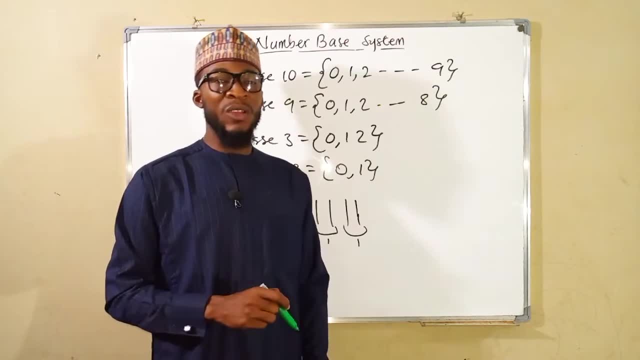 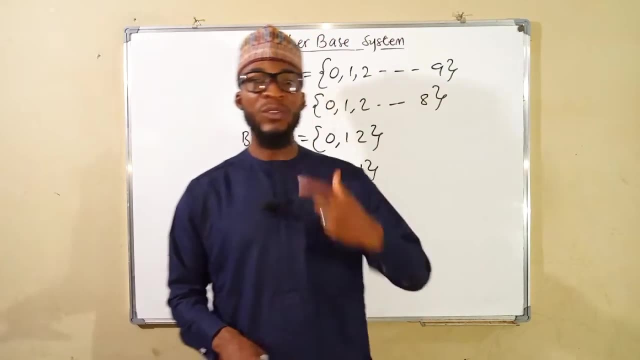 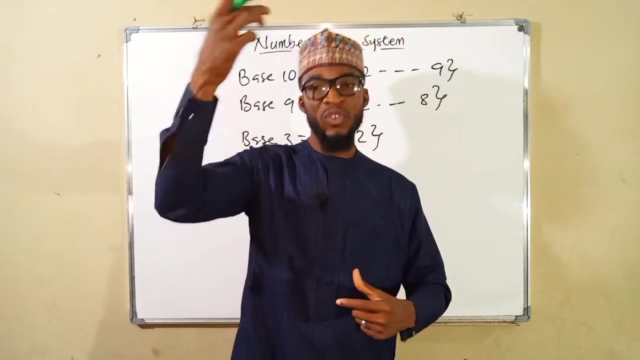 we say we have three bundles. To understand this bundle clearly, let me refer back to the numbers in base 10.. You know, naturally we count in base 10 and every time we are counting, once we reach 9,, the next number is going to be 0, because 10 is a complete. 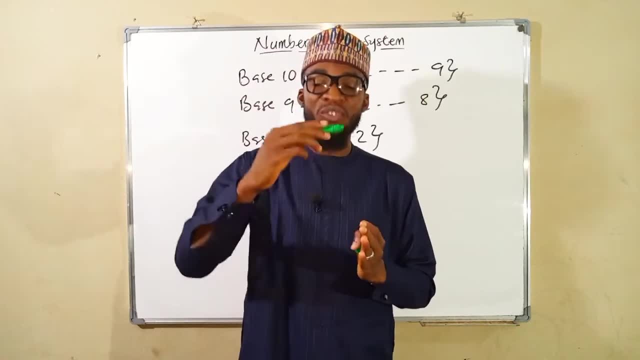 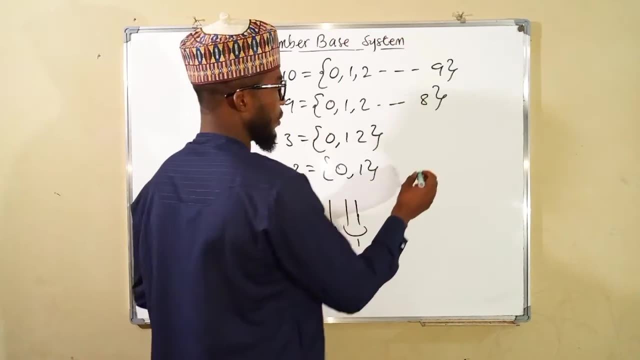 bundle And once you've completed your bundle you have to count all of our again from 0.. So suppose we have numbers like 1,, 7,, 8 in base 10.. And the second one is 6.. So the second. 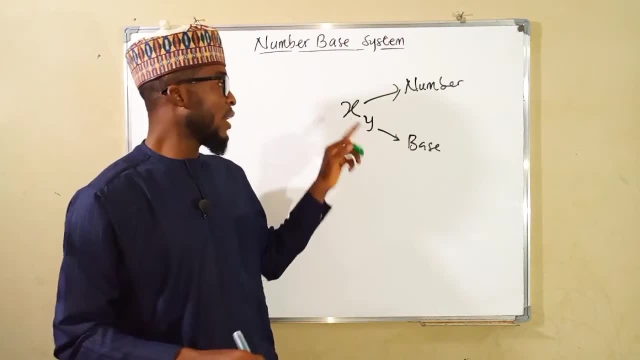 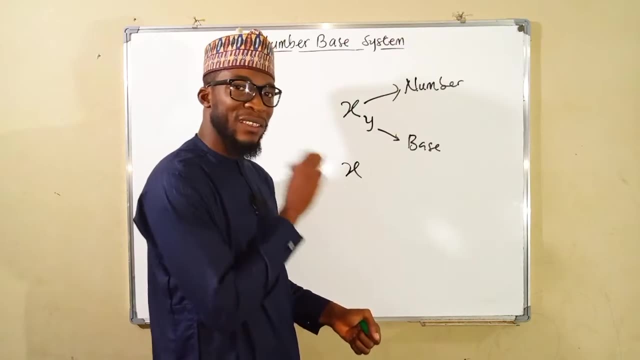 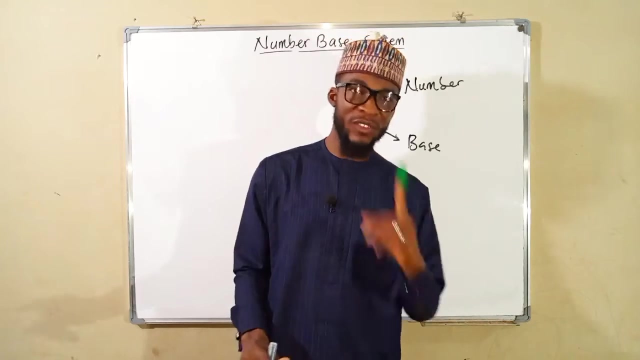 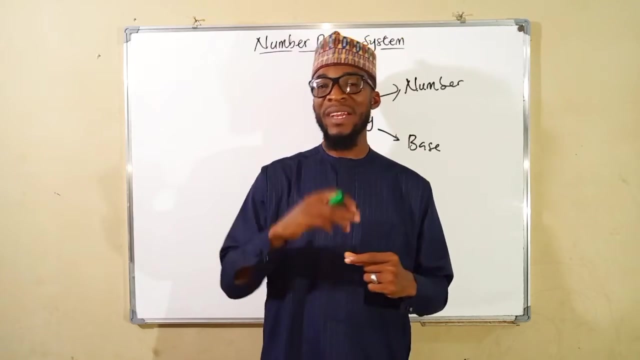 there are two important things you need to know. Any number without an assigned base- suppose we have just x as a number- If that number is in base 10, naturally if it does not contain any assigned base. that's number one. Number two: you need to know that the highest digit in any number base is one. 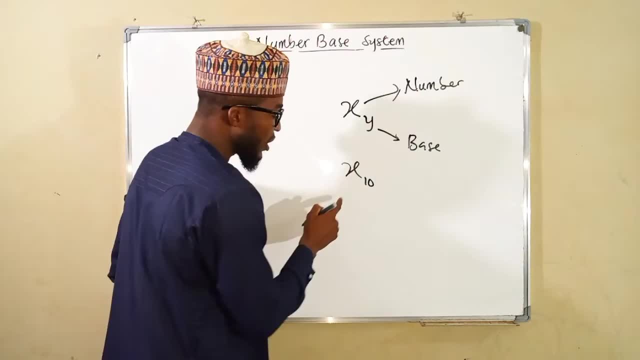 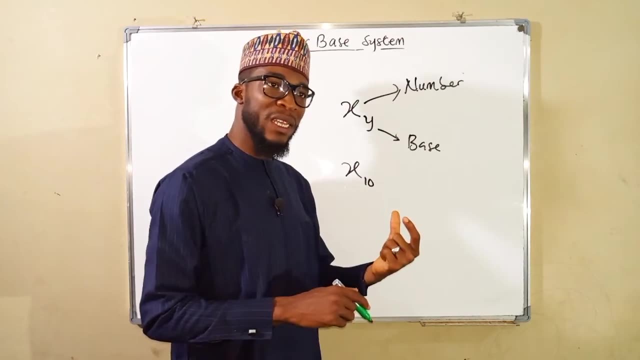 less than the base itself. So if you're talking about numbers in base 10, you'll never see 10 within the range. If you're talking about numbers in base 9, you can only see numbers from 0 to 8.. 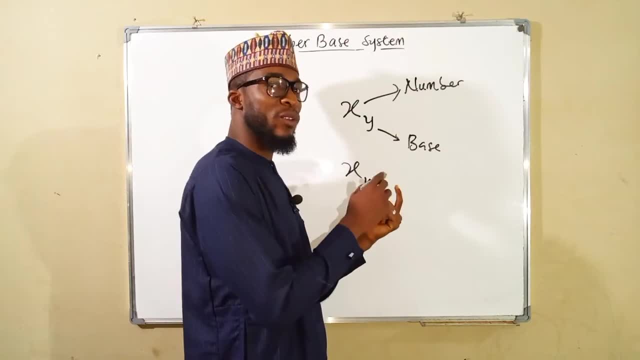 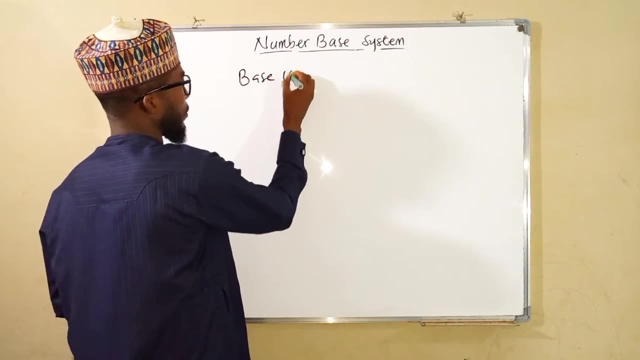 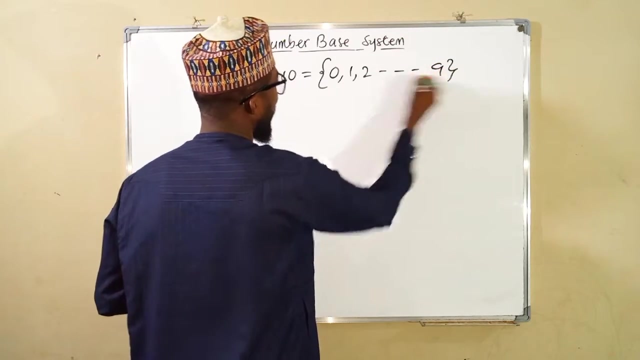 If you're base 7, you can only see numbers from 0 to 6 in that order. So for base 10, the only available numbers there are 0,, 1,, 2, up to 9.. For base 9, you can see numbers: 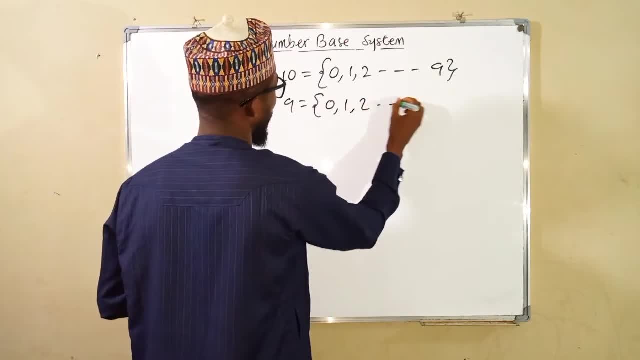 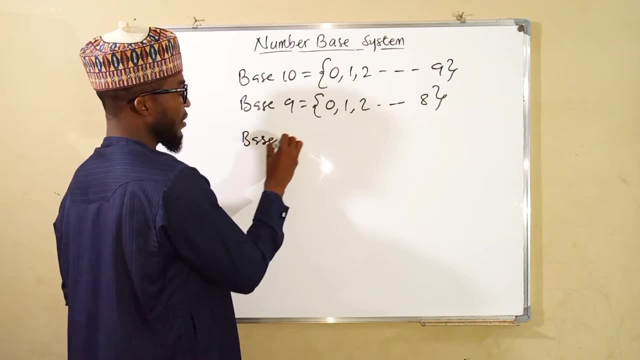 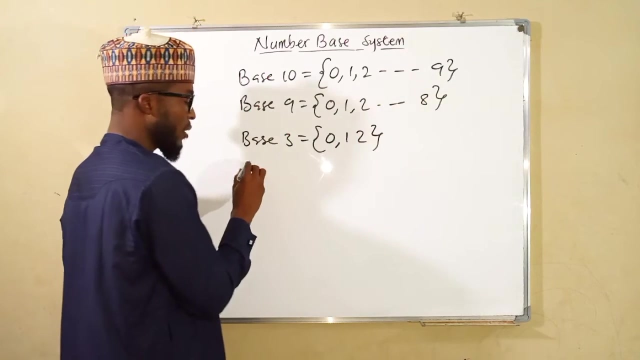 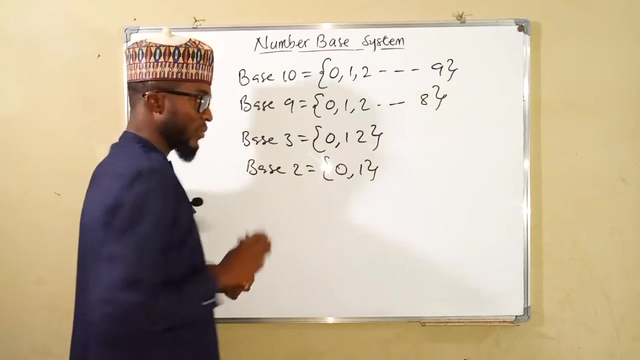 from 0,, 2, to 8.. If you're talking about base 3, you can only see numbers like 0,, 1, and 2.. If you're talking about base 2, you can only see 0 and 1.. So now let me explain. 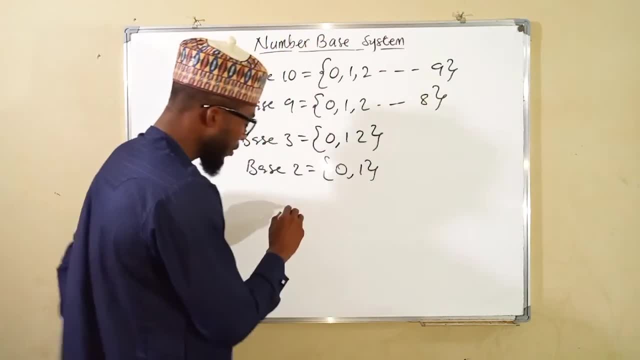 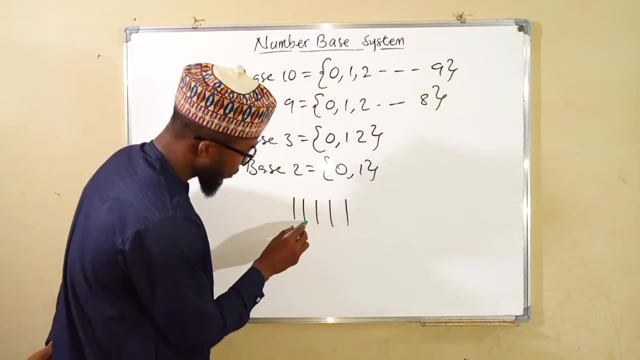 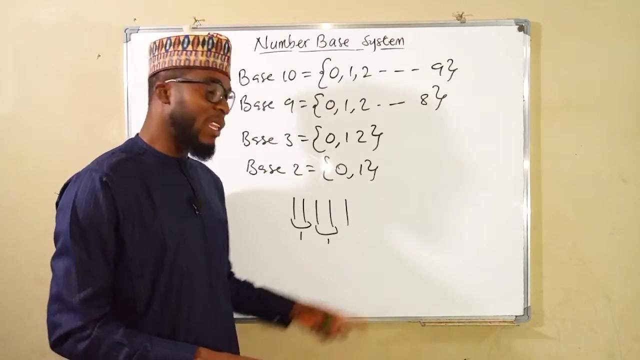 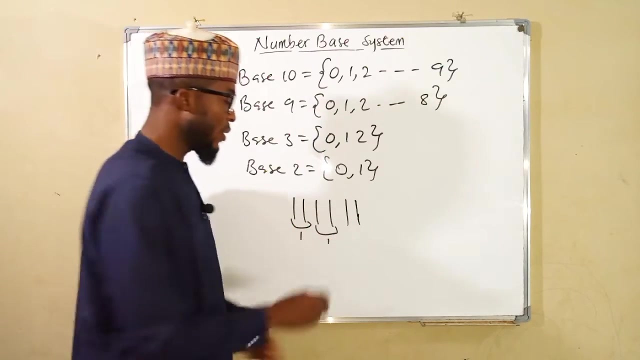 that bundle. Suppose we have five items and we want to group them in two. So every two form a bundle, every two form a bundle and we have an extra which we call a unit. And if you were to add an extra item, just a single item, that single item is going to be linked off with the unit left to form. 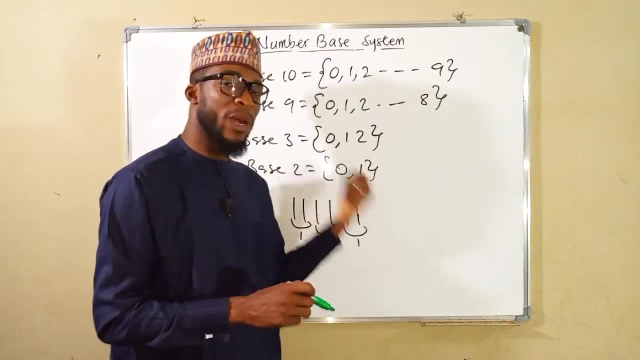 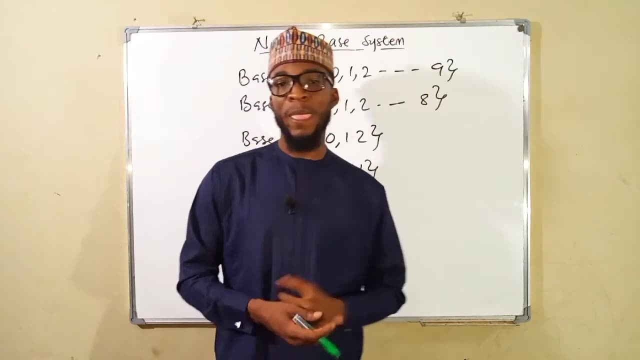 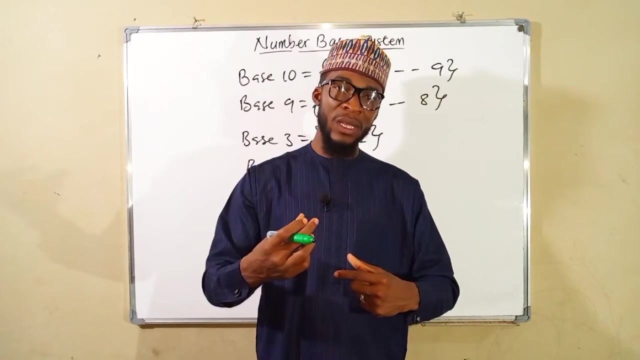 a complete bundle And hence we say we have three bundles. To understand this bundle clearly, let me refer back to numbers in base 10.. You know, naturally we count in base 10.. And every time we are counting, once we reach 9, the next number is going to be 0, because 10 is. 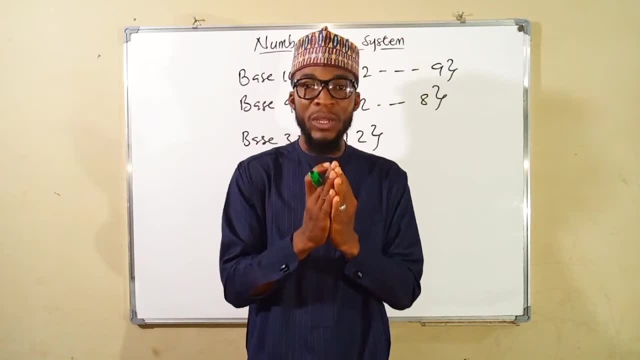 a complete bundle And once you've completed your bundle you have to recount all over again from 0.. So suppose we have numbers like 1, 2, 3,, 4,, 5,, 6,, 7,, 8, 9, 10,, 11,, 12,, 13,, 14,, 15,, 16,, 17,. 18,, 19,, 20,, 21,, 22,, 23,, 24,, 25,, 26,, 27,, 28,, 29,, 30,, 31,, 32,, 33,, 34,, 35,, 36,, 37,, 38,. 39,, 40,, 40,, 41,, 42,, 43,, 44,, 45,, 46,, 47,, 49,, 40,, 41,, 42,, 43,, 44,, 45,, 46,, 47,, 49,, 41,, 42,. 45,, 46,, 47,, 49,, 42,, 43,, 45,, 46,, 47,, 49,, 42,, 44,, 45,, 46,, 47,, 49,, 42,, 45,, 46,, 47,, 49,. 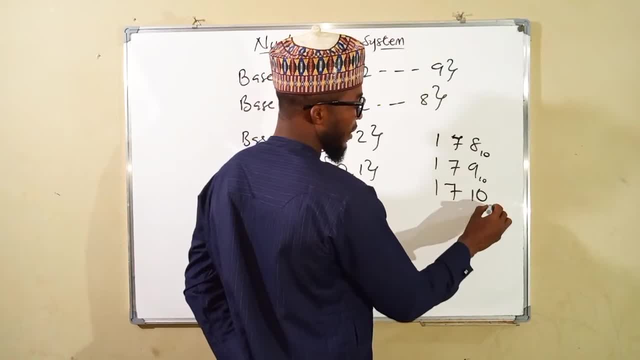 The next number is going to be 1,, 7,, 9,, also in base 10.. The next number is going to be 1,, 7,, 10 in base 10.. But remember I told you, the highest digit in any number base is 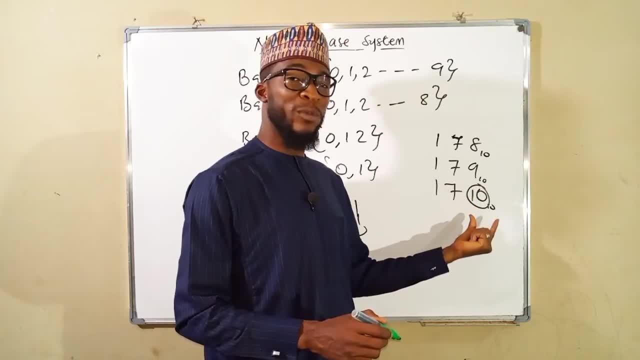 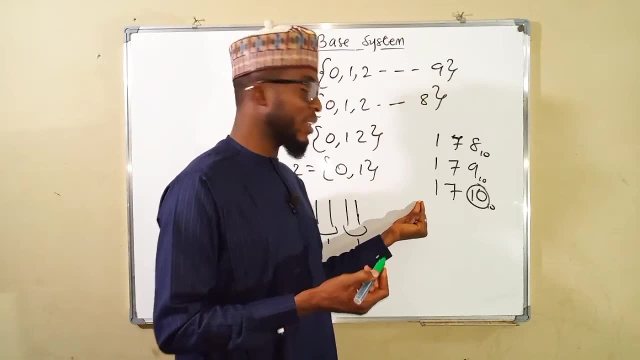 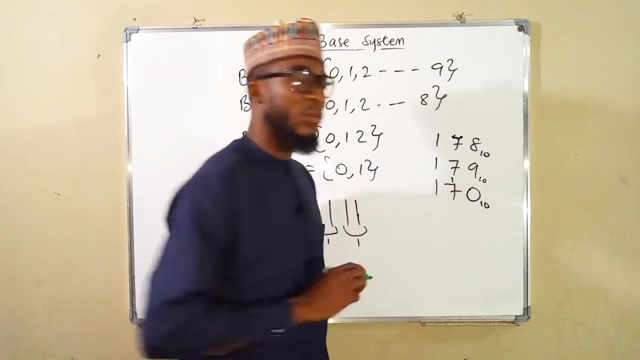 1 less than the base itself. So 10 is a complete bundle And hence you have to count all the values. you need to recount all over again from 0 and take that bundle, complete bundle- to the next number And instead of having 10 here, we have 0 is 10 and that completed. 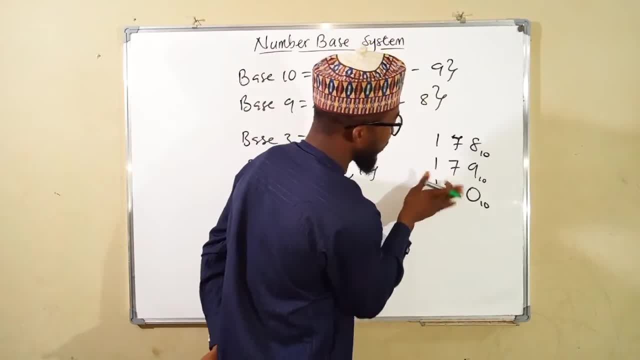 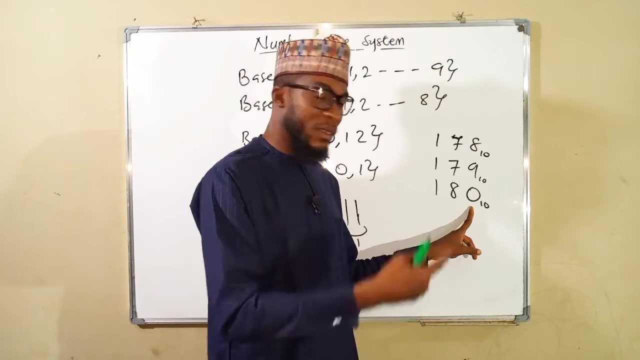 bundle should be taken to the next number and it becomes 8.. So this is bundle for you, This is unit. Unit will keep on increasing till it reaches the highest number which we have here as our base, And it will complete the bundle. 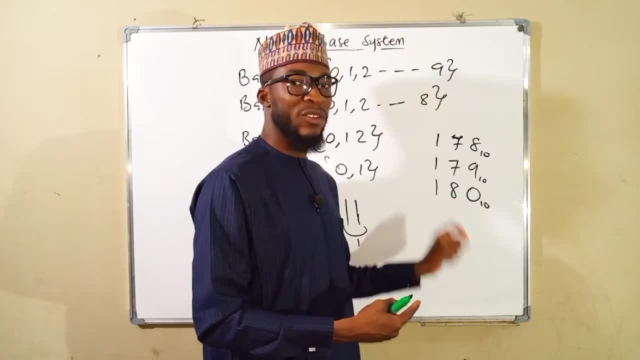 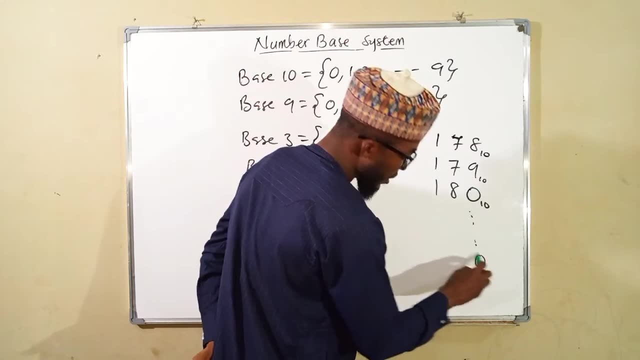 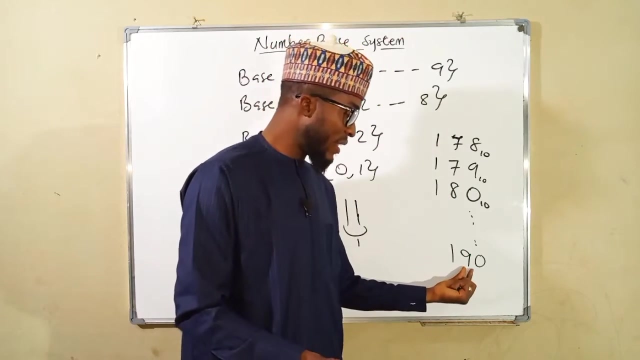 And that bundle is going to be taken to the next number. This is how it will keep on increasing till it reaches 10 again. You count all over again from 0 and this number becomes 9.. And once this next number becomes 10, it will count from 0 again and take that bundle to. 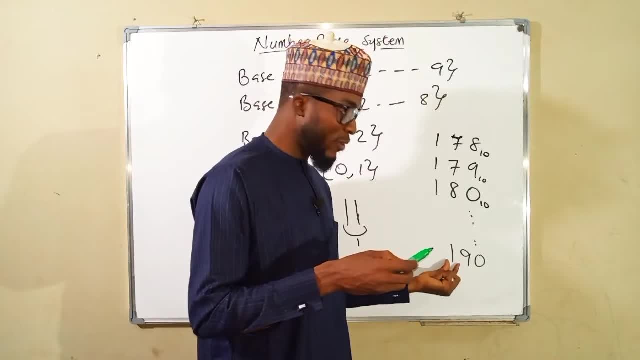 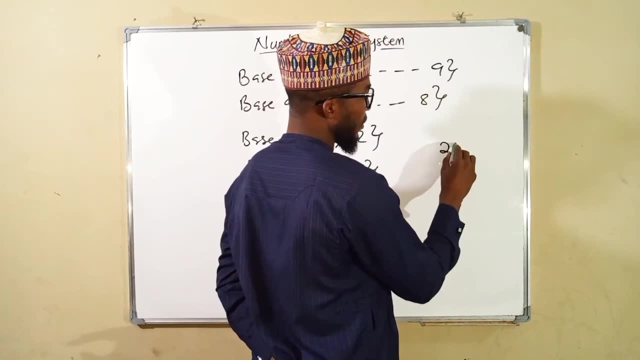 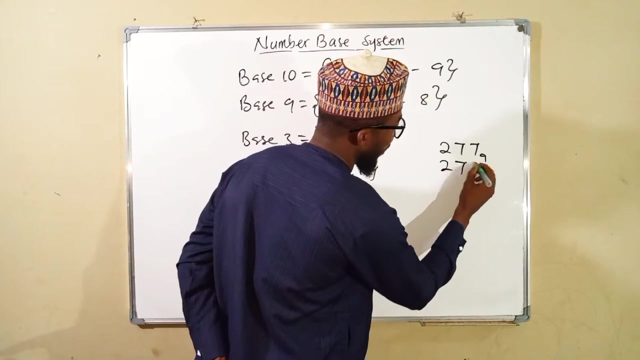 the next. So units form bundles and bundles form other bundles. For base 9, suppose we have 2,, 7,, 7, base 9.. The next number is going to be 2,, 7,, 8, base 9.. 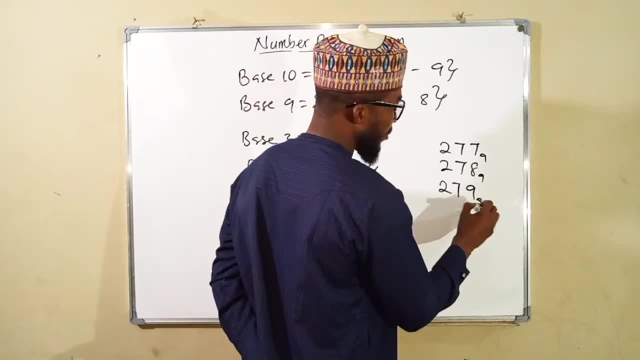 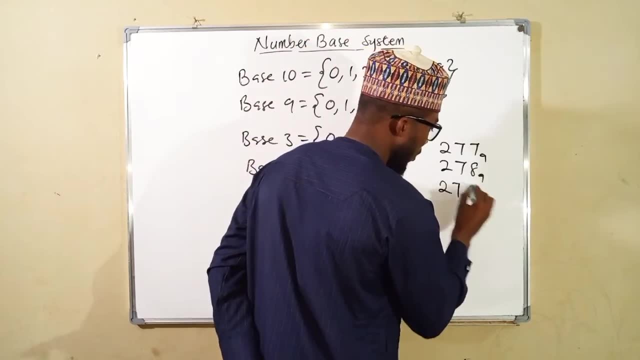 The next number, 2,, 7,, 9,, base 9.. But we do not have 9.. 9 is a complete bundle, So instead of writing 9,, we write 0. And we take that bundle to the next And this becomes 8.. If you keep. 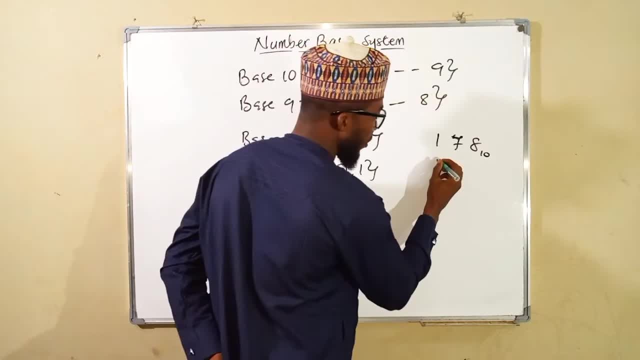 number is 7.. And the first number is 8. And the first number is 9.. All right, So let me notice one thing here. Let's look at this, Let's see if that really makes sense for me. You know, the next number is going to be 179, also in base 10.. 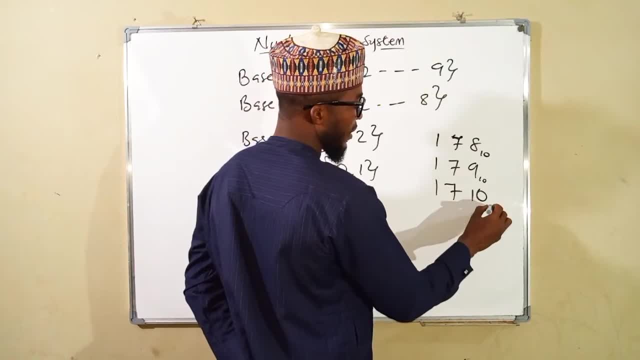 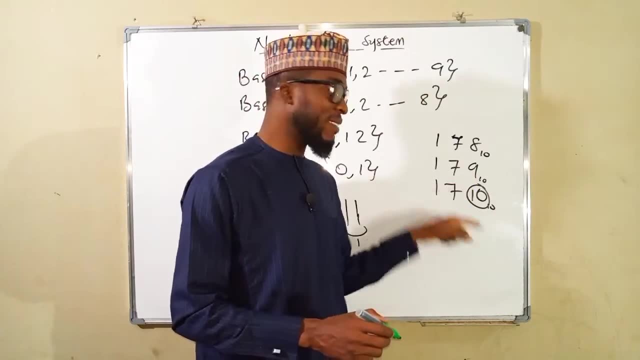 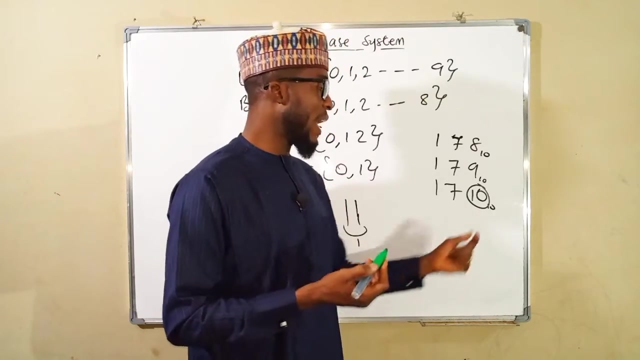 The next number is going to be 1710 in base 10, but remember I told you, the highest digit in any number base is 1 less than the base itself. So 10 is a complete bundle and hence you need to recount all over again from 0 and take. 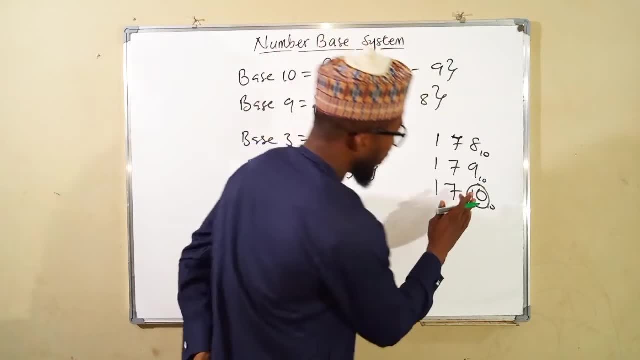 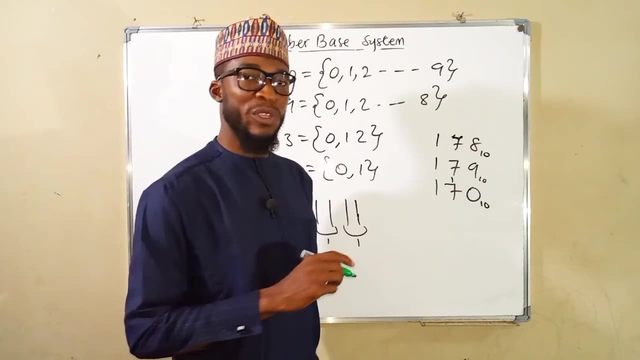 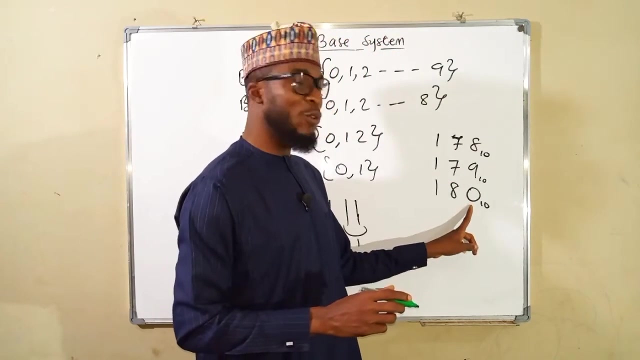 that bundle, complete bundle, to the next number And instead of having 10 here we have 0 is 10, and that completed bundle should be taken to the next number and it becomes 8.. So this is bundle for you, this is unit. 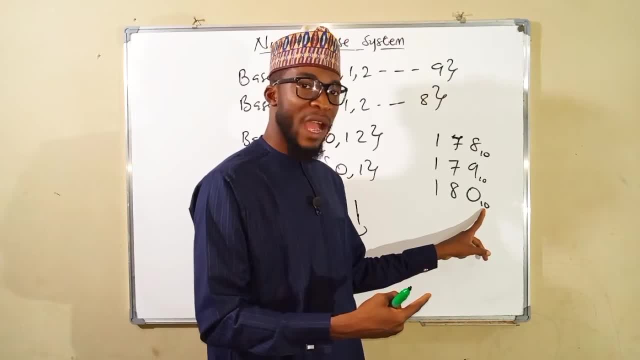 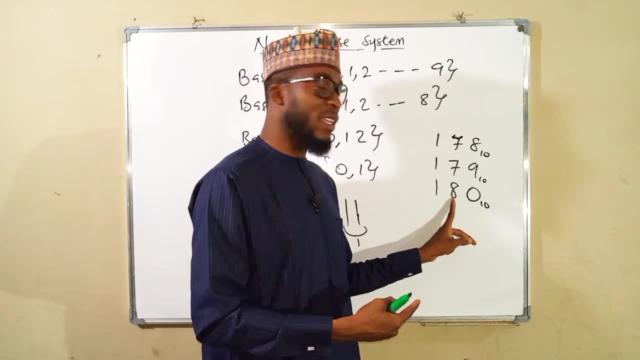 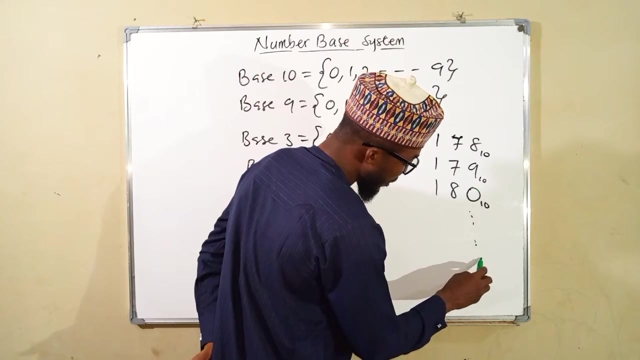 Unit will keep on increasing till it reaches the highest number which we have here as our base, and it will complete a bundle and that bundle is going to be taken to the next number. This is how it will keep on increasing Till it reaches 10 again. you count all over again from 0 and this number becomes 9.. 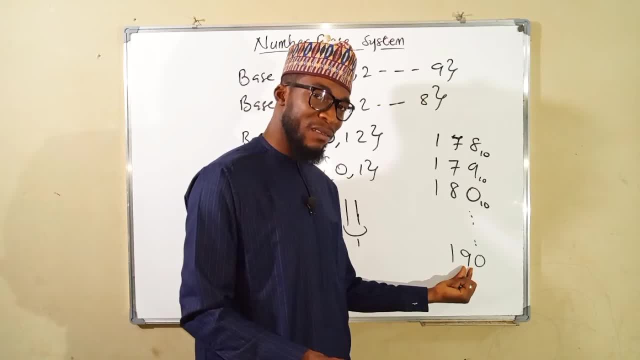 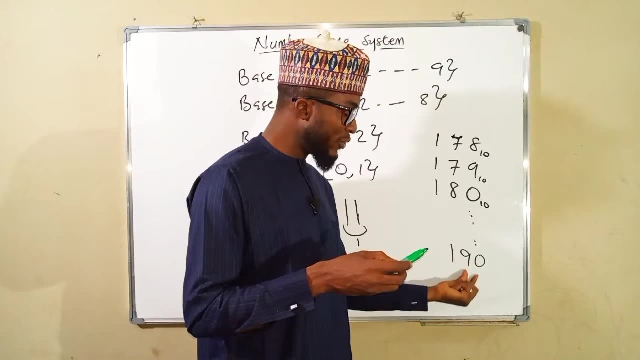 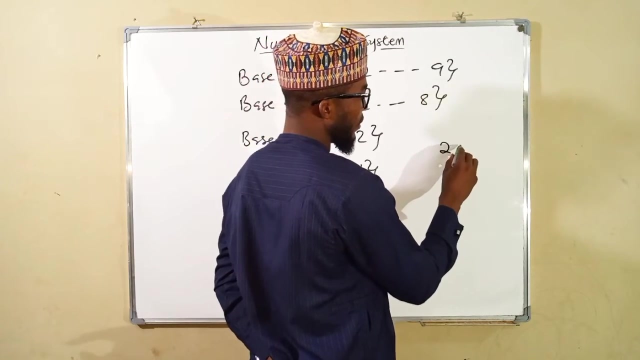 And once this next number becomes 10, it will count from 0 again and take that bundle to the next. So units form bundles and bundles form other bundles For base 9.. Suppose we have 2,, 7,, 7,, 9.. 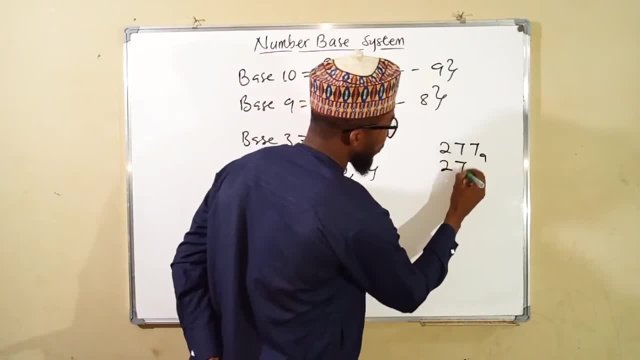 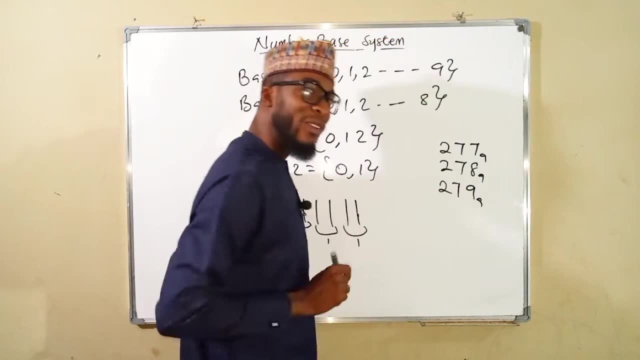 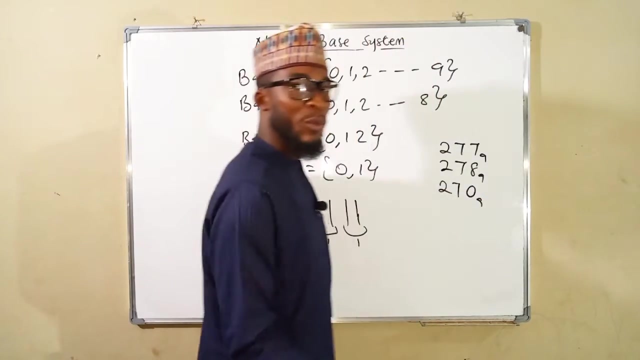 Base 9.. The next number is going to be 2, 7, 8, base 9.. The next number: 2, 7, 9, base 9.. But we do not have 9.. 9 is a complete bundle, so instead of writing 9, we write 0 and we take that bundle to the 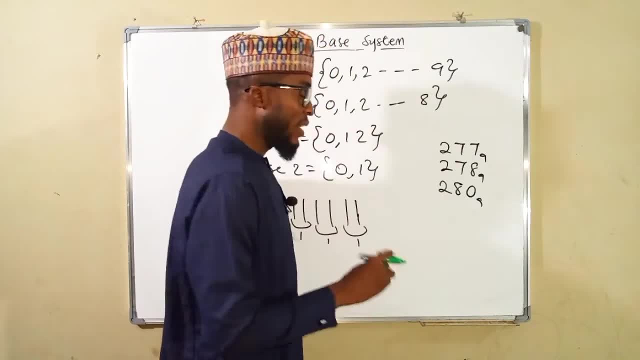 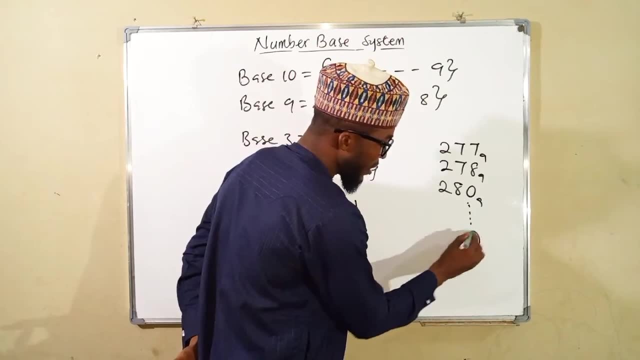 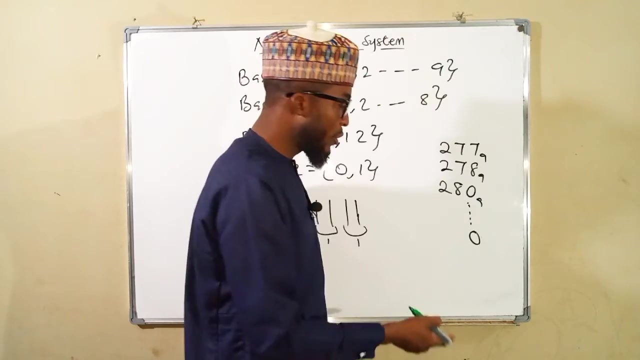 next and this becomes 8.. If you keep on increasing this till it reaches 9, it becomes 0 again and it will take that bundle to the next. And if you take that 1 to the next, it becomes 9, and 9 is a complete bundle and you have to. 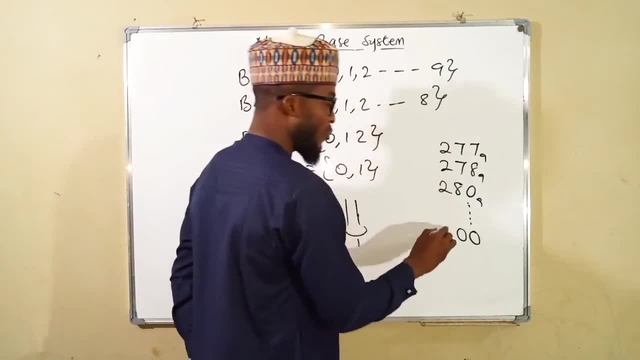 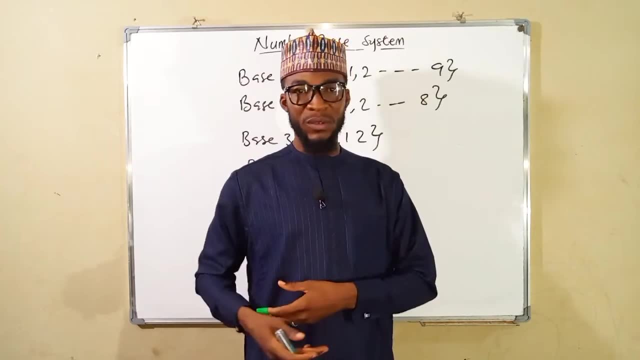 write 0 again and take that bundle to the next and it becomes 3. Base 9. Now in base 2 you can only see zeros and ones, which is also very essential in computing. You know, computers only understands zeros and one. 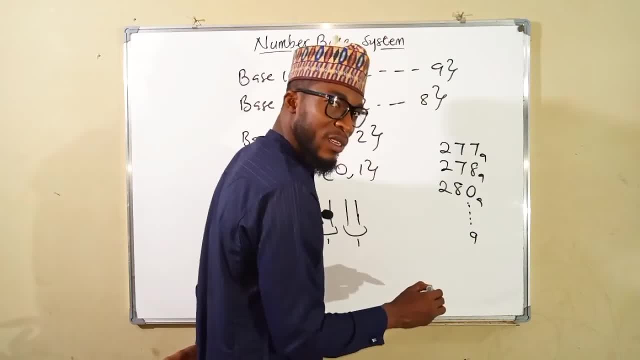 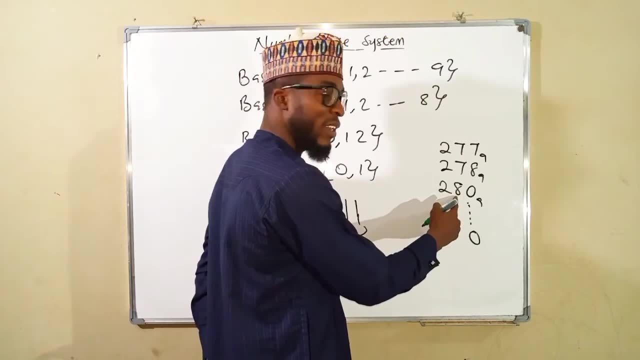 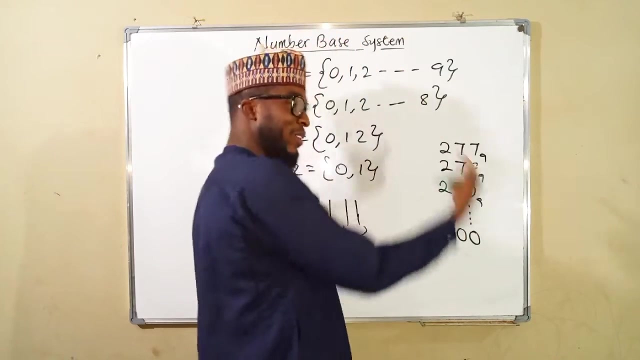 on increasing this till it reaches 9, it becomes 0 again And it will take that bundle to the next, And if you take that one to the next, it becomes 9.. And 9 is a complete bundle And you have to write 0 again And take that bundle to the next And it becomes 3.. Base: 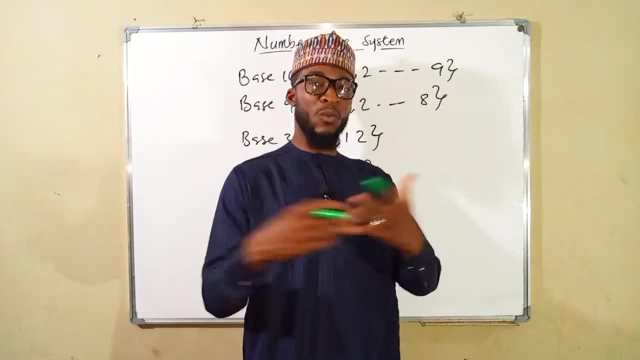 9. Now in base 2, you can only see 0s and 1s, which are also very essential in computing. You know computer only understands 0s and 1s, So you can only see 0s and 1s. So you 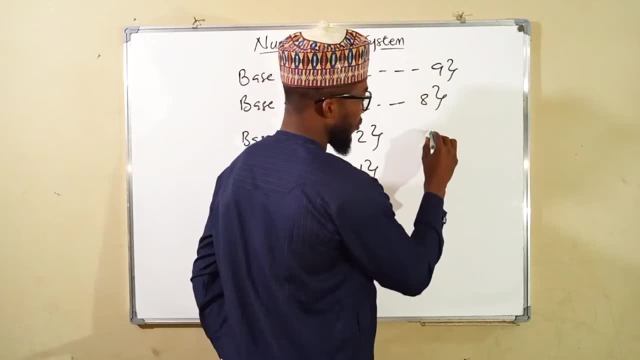 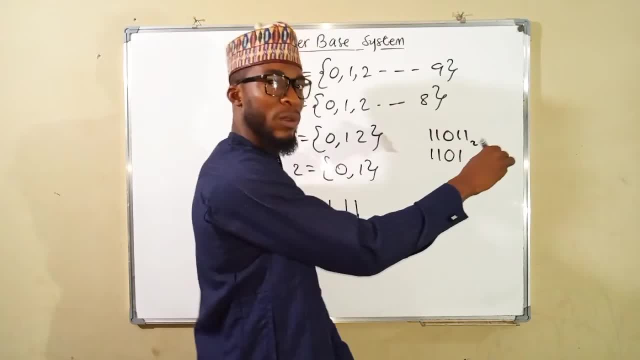 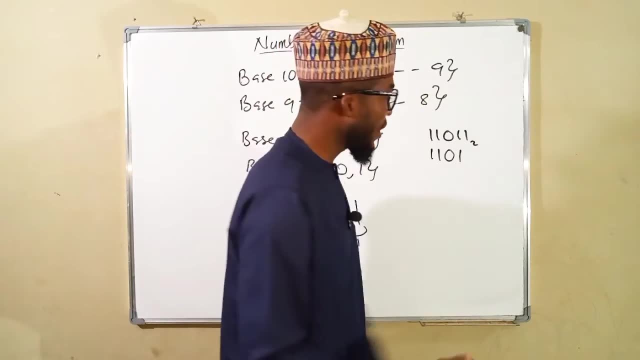 number is going to be 1, 1, 0, 1, 2.. But you can never write 2 in base 2.. 2 is a complete bundle. Then you write the remainder, which is 0. And you take that bundle to the next. 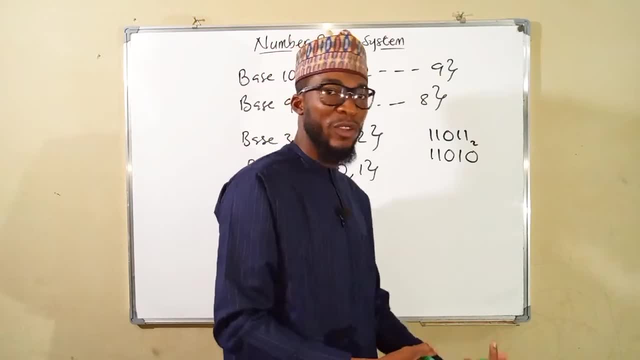 And this also becomes 2.. And once it becomes 2, it is a complete bundle. You have to write 0. And take that 1 to the next, And this becomes 1.. And this becomes 2.. And once it becomes 2, it is a complete bundle. You have to write: 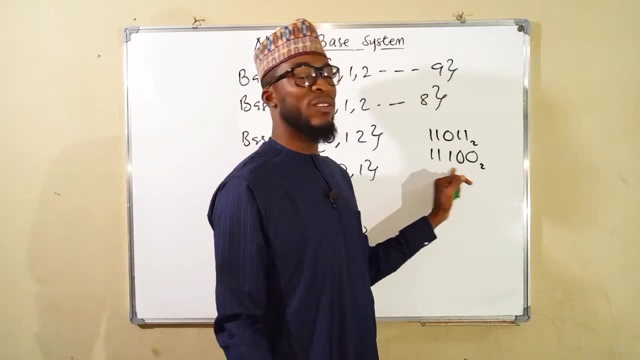 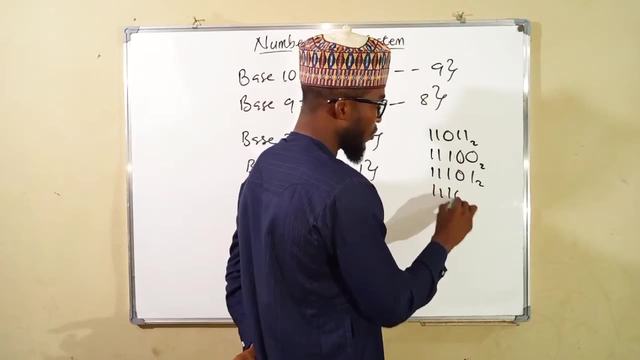 1.. So the next number after this is 1, 1, 1, 0, 0.. Next number: 1, 1, 1, 0, 1 is 2.. Next number: 1, 1, 1, 0.. This becomes 2.. Complete bundle. You write 0.. You take that bundle. 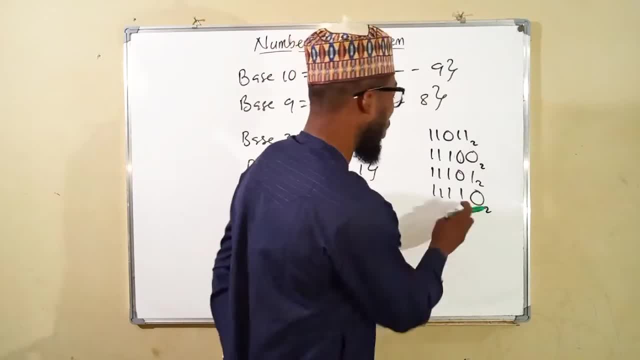 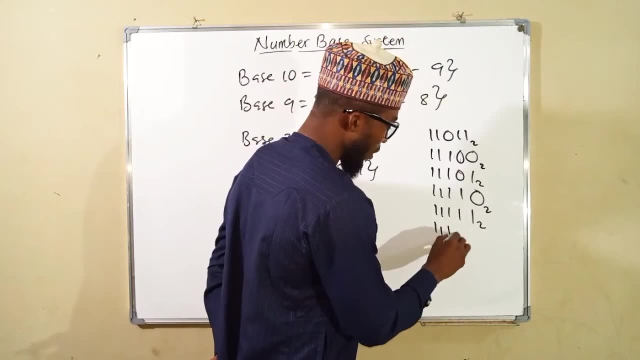 to the next, And this becomes 1.. Next number: 1, 1, 1, 1, 1.. The next number: 1, 1, 1, 1.. Instead of 2,, you write 0.. 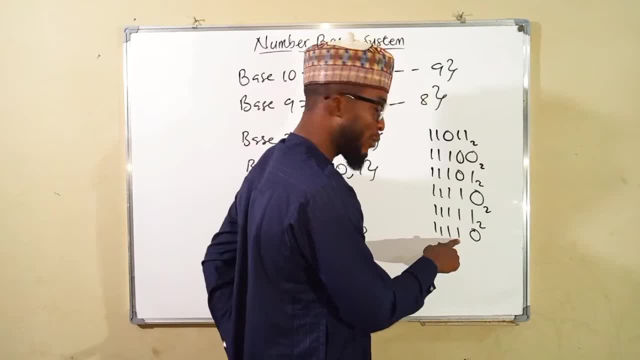 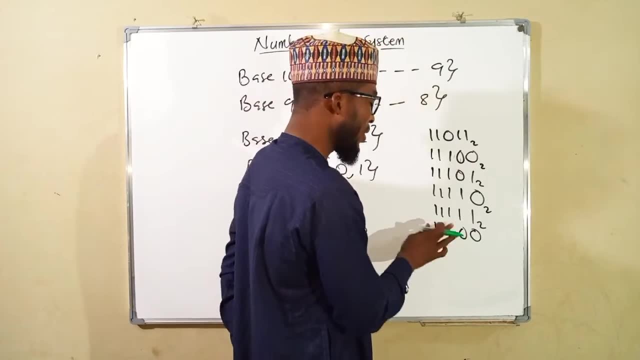 And take that 1 to the next, It becomes 2 again. Complete bundle. You write 0.. You take that 1 to the next. 1 plus 1, 2, it becomes a complete bundle. You write 0. You take it. 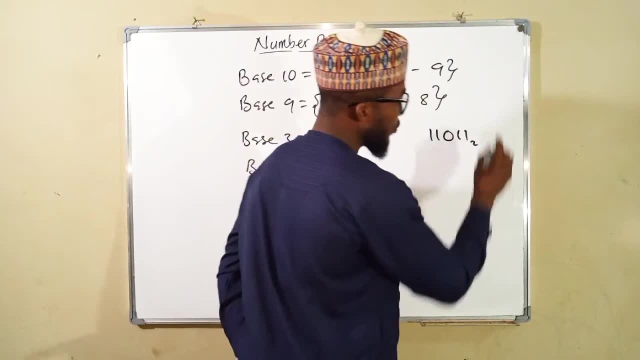 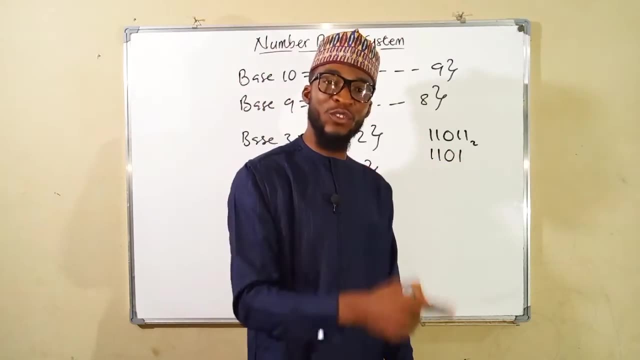 Suppose we have 0, 1, 1, 0, 1, 1 in base 2.. State index, index, Date index, nil going to be 1 1, 0, 1, 2, but you can never write 2 in base 2.. 2 is a complete bundle. 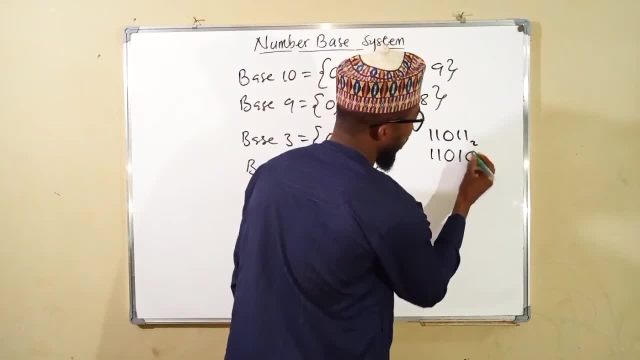 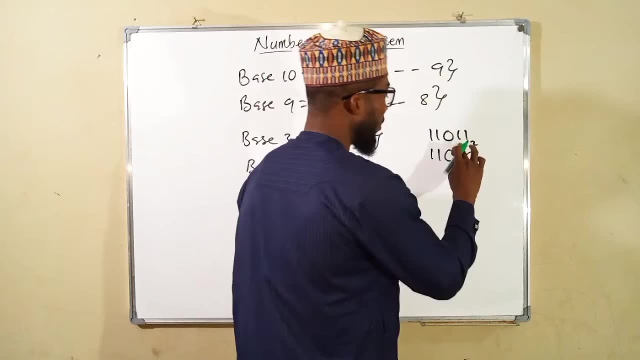 then you write the remainder, which is 0, and you take that bundle to the next and this also becomes 2, and once it becomes 2, it is a complete bundle. you have to write 0 and take that 1 to the next and this becomes 1. so the next number after. 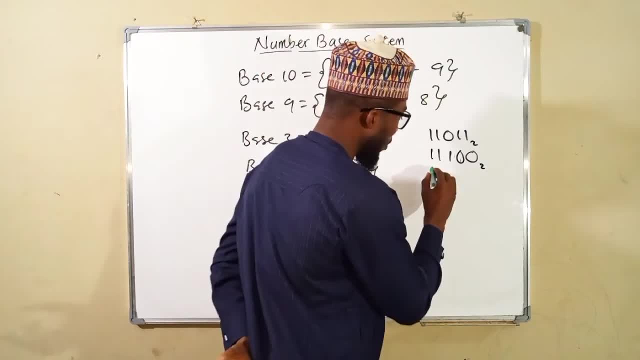 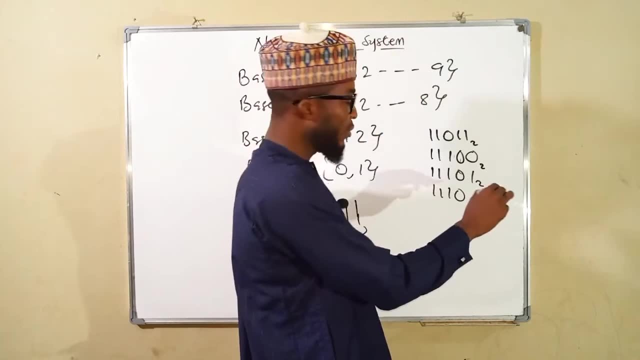 this is 1 1 1 0 0. next number: 1 1 1 0. 1 is 2. next number: 1 1 1 0. this becomes 2. complete bundle. you write 0, you take that bundle to the next and this becomes: 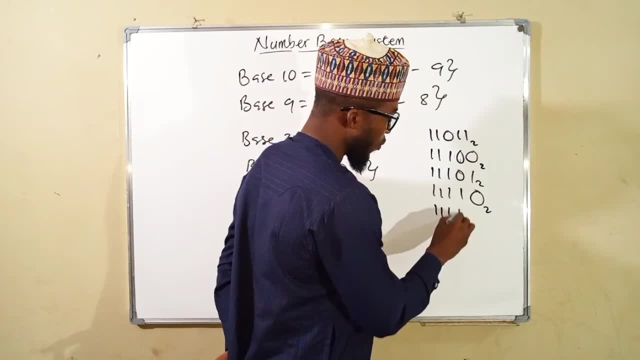 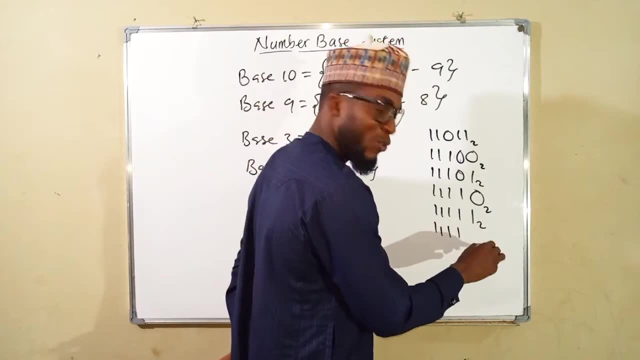 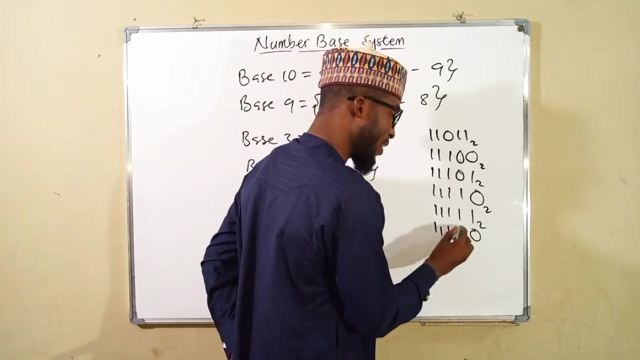 1. next number: 1, 1, 1, 1, 1. the next number: 1, 1 1, 1 instead of 2. you write 0 and take that 1 to the next. it becomes 2 again, complete bundle. you write 0. you take that 1 to the next 1. 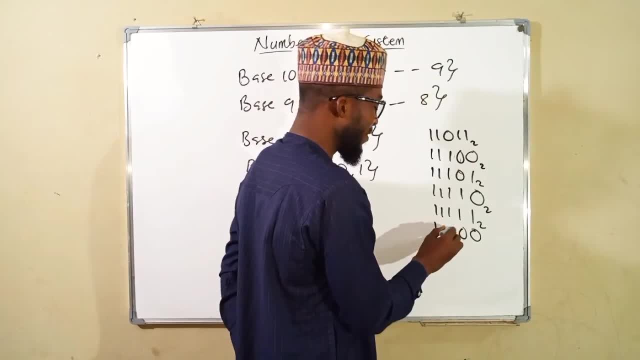 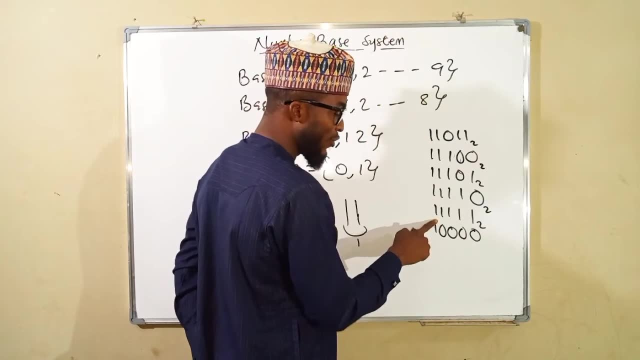 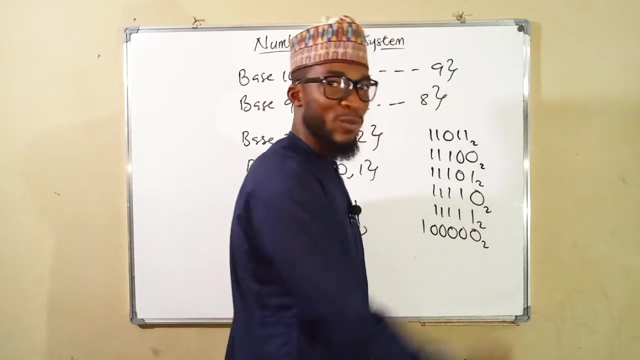 plus 1, 2, it becomes a complete bundle. you write 0, you take it to the next, it becomes 2. you write 0, you take it to the next, it becomes 2. you write 0, you take that 1 to the next and you have 1, 0, 0, 0, 0, 0. base 2: this is the next number. so 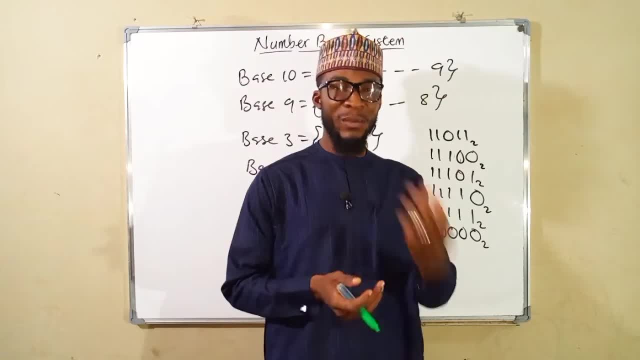 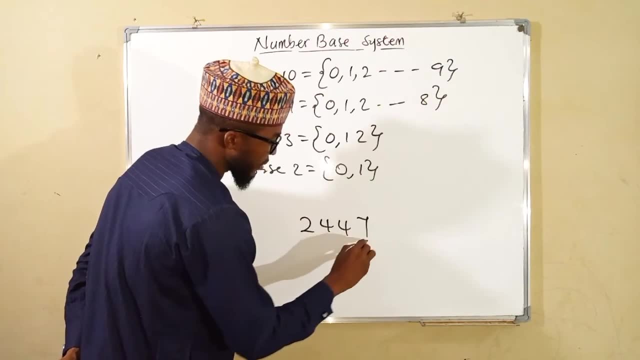 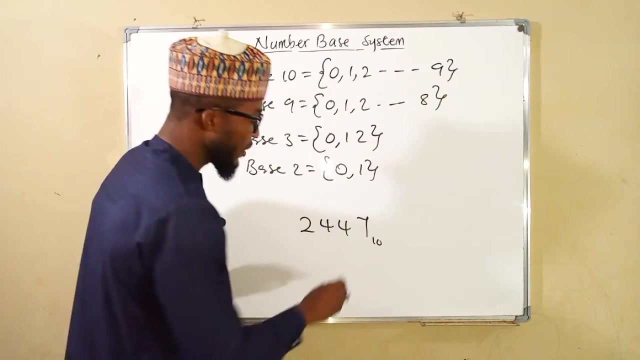 that's something which is very important again in elementary school, In elementary arithmetics, base 10. suppose we have 2, 4, 4, 7 in base 10. you know naturally the last number or the last digit. we call it unit because unit is. 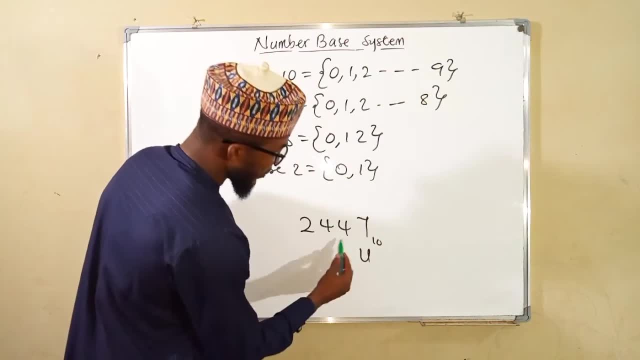 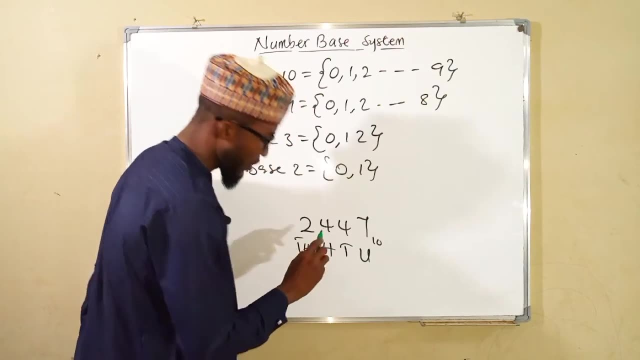 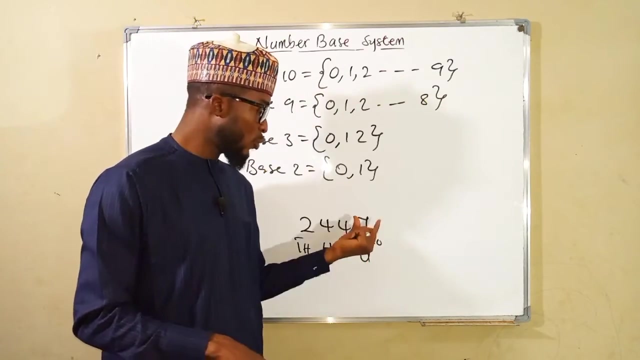 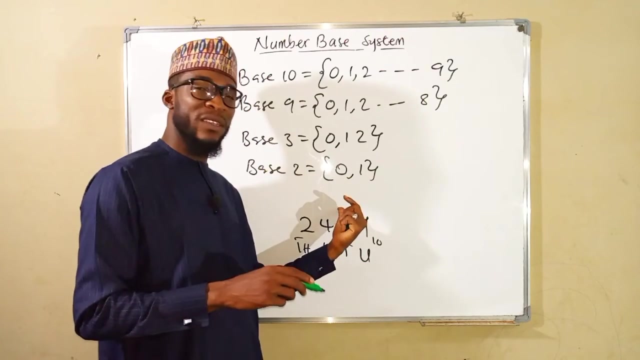 the first value of 7 here and the next before it. we call it tens, hundreds and thousands. why do we have this place values? remember we are counting in base 10, so once 7 reaches 10, to count all over again for a 0. and take that bundle to the next number, which is 4 here, to make it. 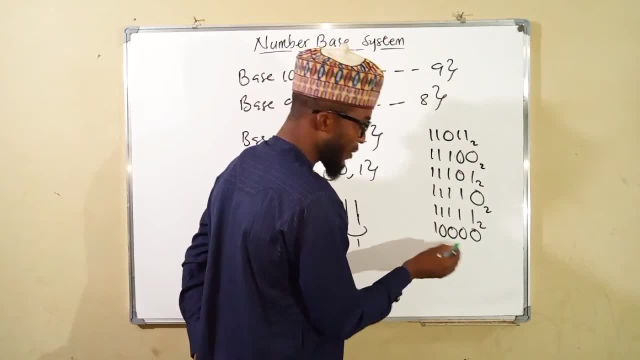 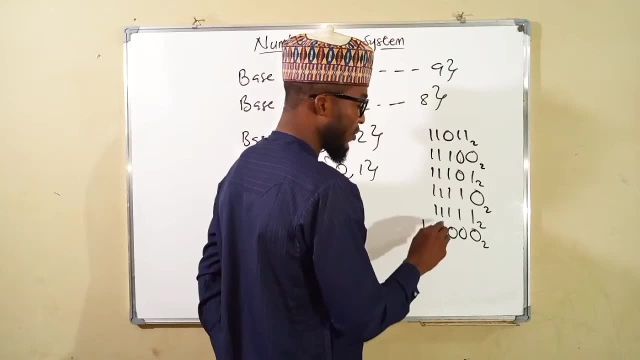 to the next, It becomes 2.. You write 0.. You take it to the next, It becomes 2.. You write 0. You take that 1 to the next And you have 1, 0, 0, 0, 0, 0, base 2.. This is the next. 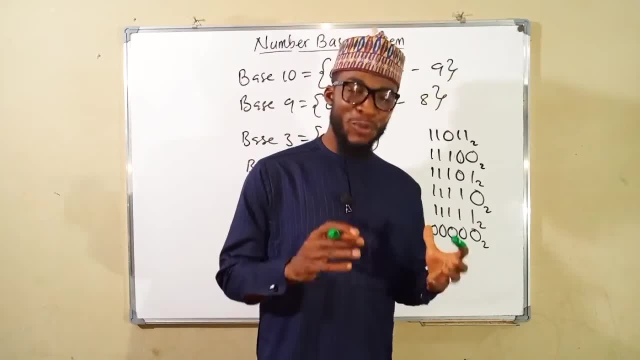 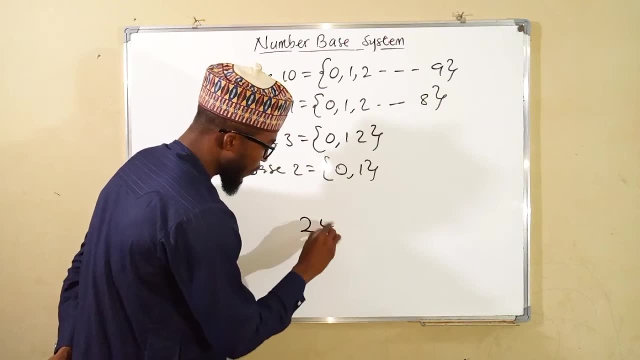 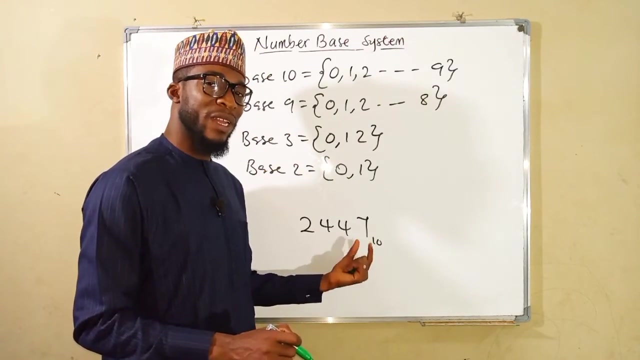 number. So that's something which is very interesting, important again in elementary arithmetics, base 10.. Suppose we have 2, 4,, 4,, 7 in base 10.. You know naturally the last number or the last digit. 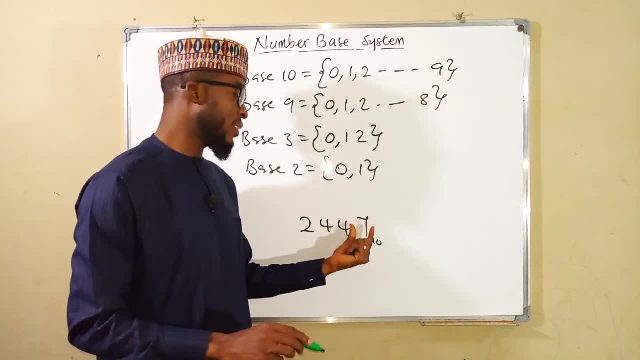 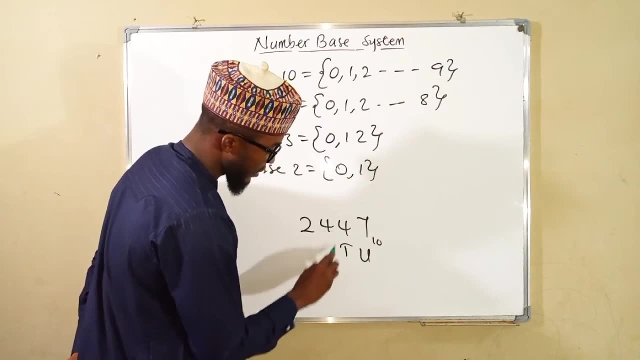 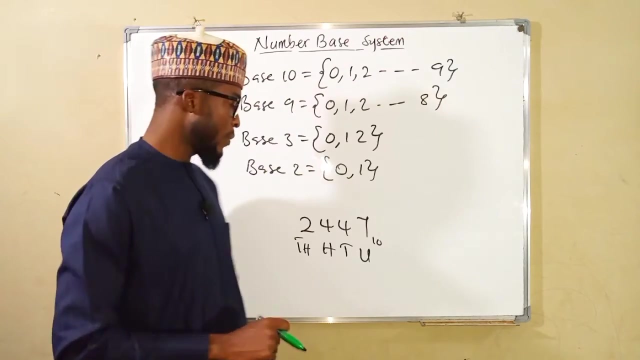 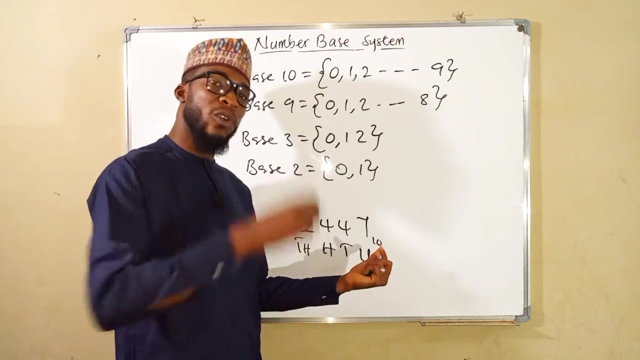 we call it unit because unit is the first value of 7 here And the next before it. we call it tens, hundreds, and thousands. Why do we have this place values? Remember, we are counting in base 10.. So once 7 reaches 10, it will count all over again for a 0. 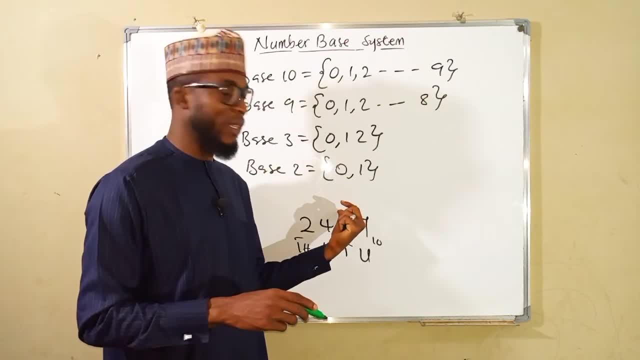 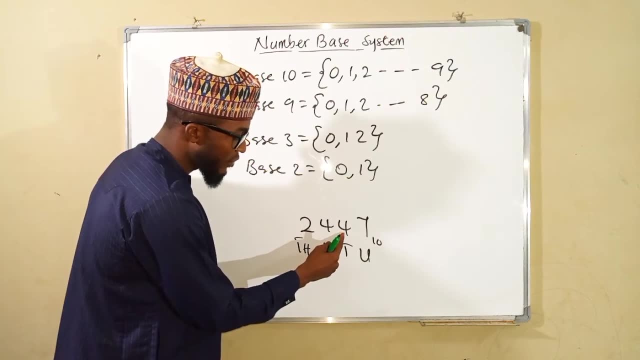 and take that bundle to the next number, which is 4 here to make it 5.. So every 10 rounds give the next number a chance to move. Every 10 rounds will give the next number a chance to move. So this is 10.. 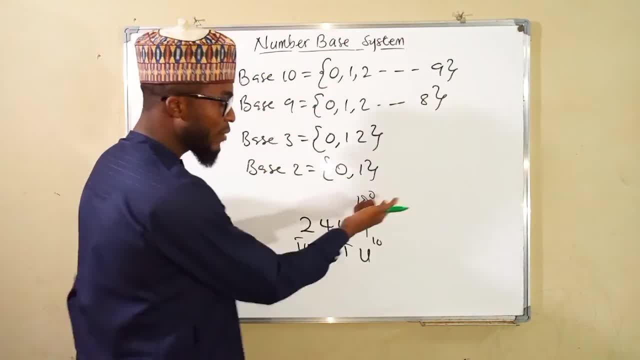 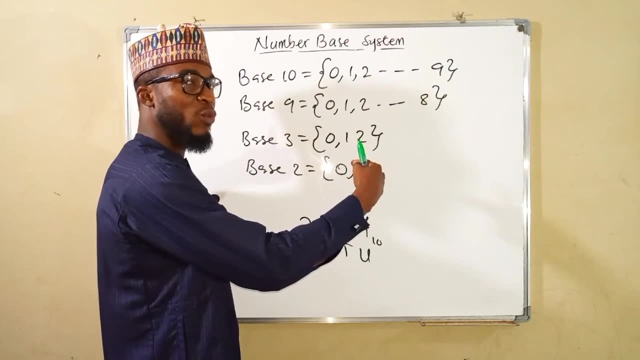 10 power 0, if we are talking about unit And 10 power 0,, remember, is 1.. And 1 is the same thing as unit. 10 power 0 is 1 times 10 is 10 power 1.. 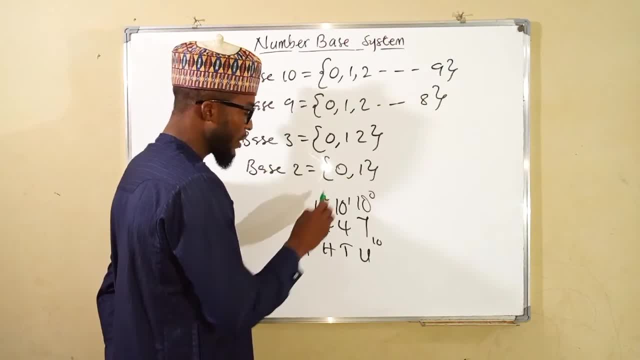 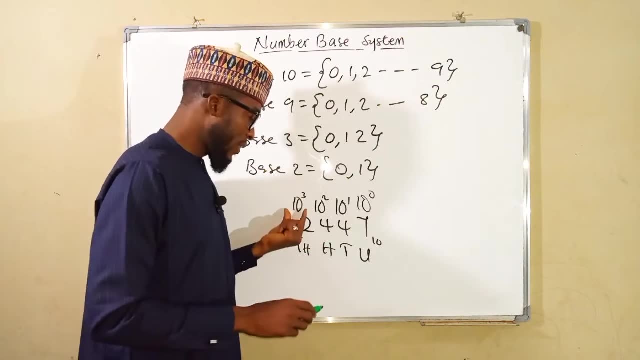 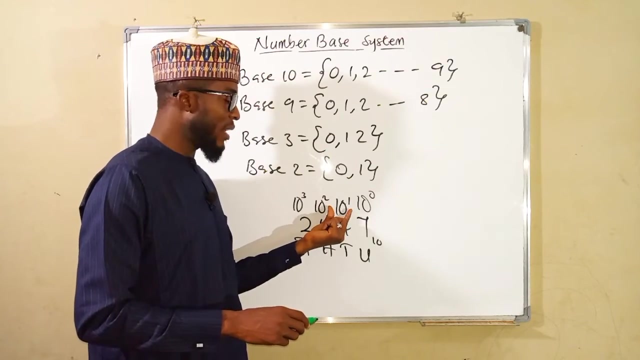 And 10 power 1 times 10 is 10 power 2.. 10 power 2 times 10 is 10 power 3. This means that this number here is 10 times as significant as this. This one is 10 times as significant as this. 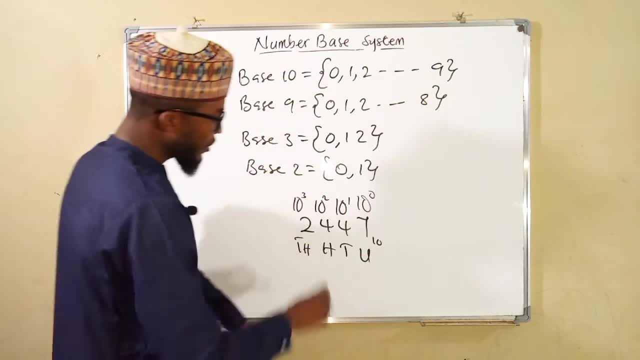 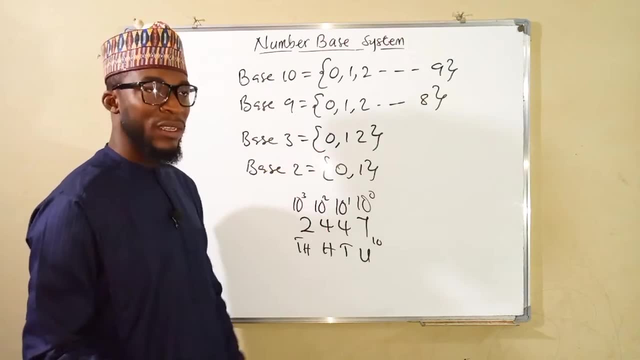 And this other one is 10 times as significant as this. So now let us simplify this: 10 power 0 is 1.. This is why we have a unit. 10 power 1 is 10.. This is why we have tens here. 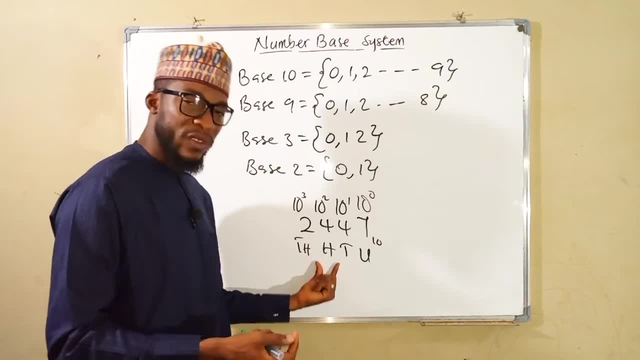 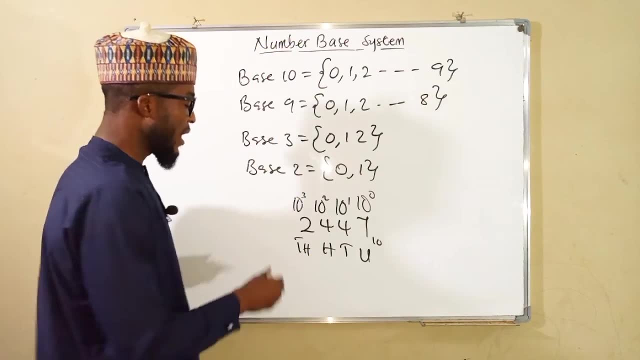 10 power 2 is 10 times 10,, which is 100.. This is why we have hundreds here. 10 power 3 is 10 times 10 times 10,, which is 1,000.. And this is why we have 1,000 here in that order.